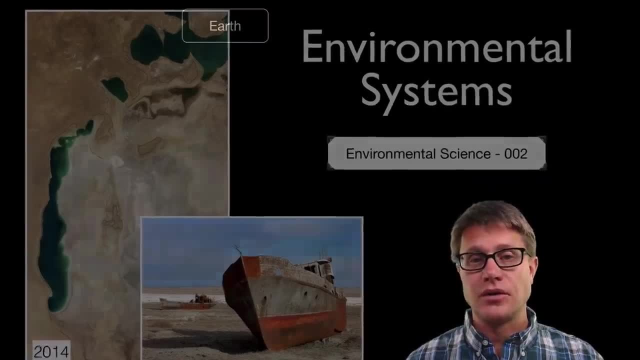 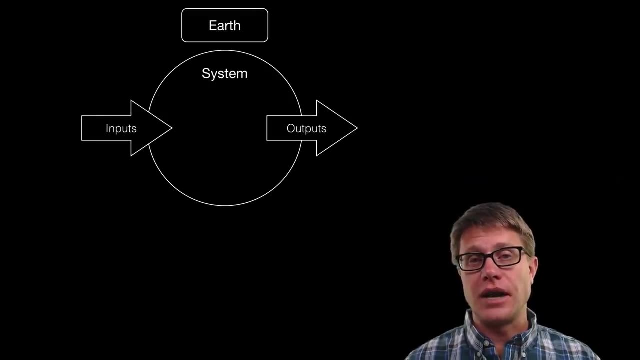 system, We were not managing the inputs and the outputs. So the earth, at the largest level, is a system. It is separated from its surroundings, And understanding the inputs and the outputs allows us to manage a system, And so the big things we are looking at are the matter and then the energy. The matter, remember, is what? 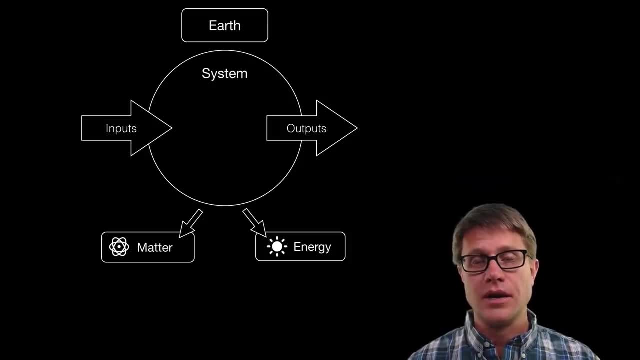 we are made of. It is the atoms that make us, and the rock and the water, And the energy is the ability to do work. Now, if we look at the matter on our planet, it is actually a closed system. The amount of matter we have on our planet is conserved. We do not get. 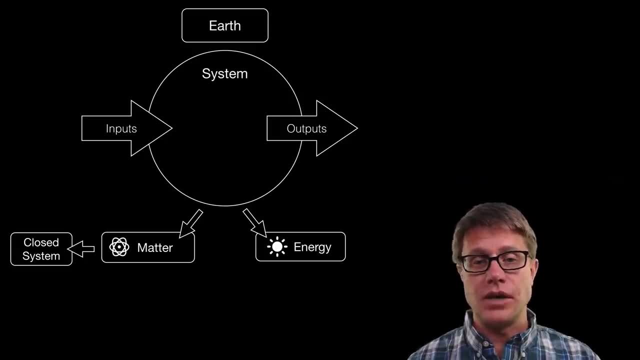 new matter from space, So we are stuck with the atoms that we have. It is conserved over time. If we look at the energy, however, it is more of an open system. We continue to get energy coming from the sun and we lose. 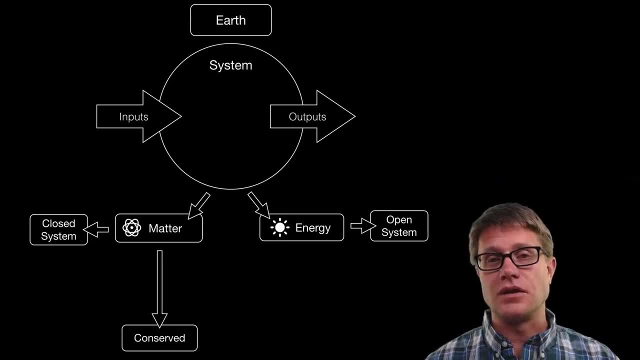 that energy as heat, And so the thing about matter you should understand is that it is conserved, And this has huge ramifications If we are looking, for example, for minerals. you cannot just grow minerals. The amount of minerals we have on our planet are finite. 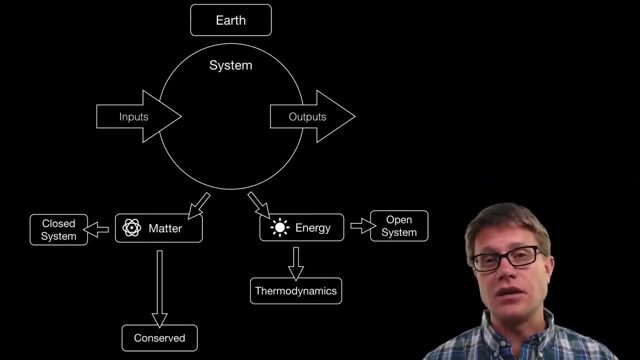 and we have to go find those minerals. If we are looking at energy, understanding the laws of thermodynamics, the first law is essentially the conservation of energy. Energy can neither be created nor destroyed. But the second law is also important And that deals with 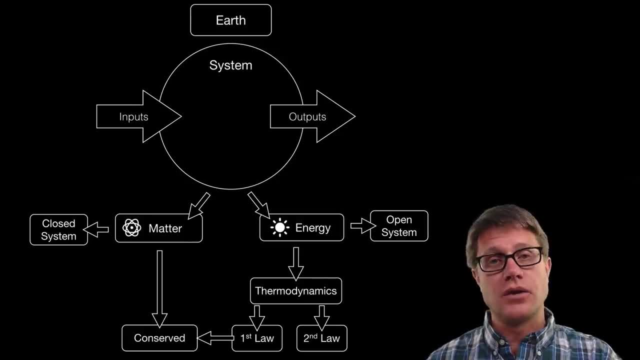 the amount of useful energy. Every time we have an interaction when we are converting energy, we are losing some of that useful energy, And so understanding how a system works is done through systems analysis. If it does not change, we say that system is at steady. 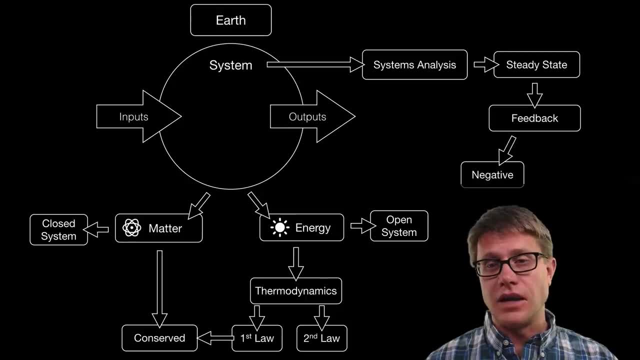 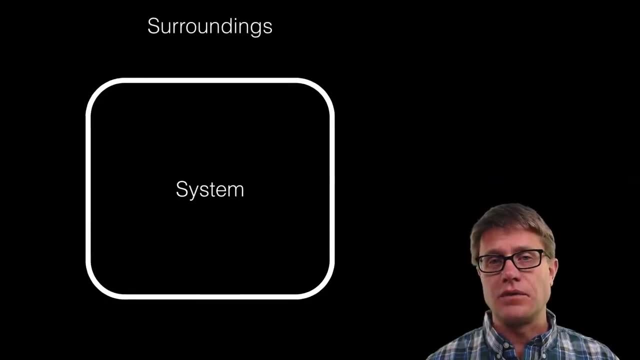 state or at equilibrium, And we can move it towards steady state using a negative feedback loop or away using a positive feedback loop. And so, big picture, a system is simply separated from its surroundings using a boundary, And we would call this a closed system, Like. 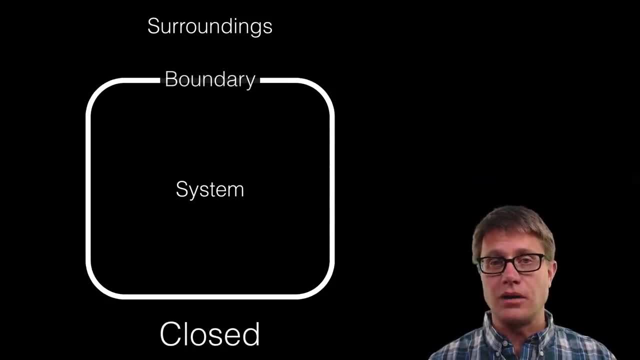 the matter we have on our planet is a closed system. We do not get new matter, We do not lose matter generally to space. If we look at an open system like energy, then there is flow from the surroundings into the system and vice versa, And so matter on our planet. 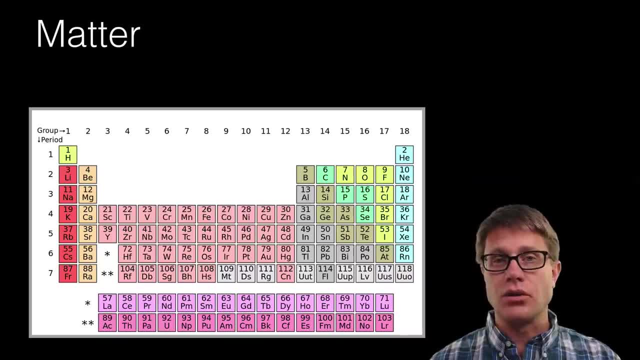 is made up of a finite amount of atoms, And atoms are organized on the periodic table. If we look at the simplest atom, hydrogen, is going to have one proton and one electron. It is highly reactive. Everything else in this column is also reactive because it has 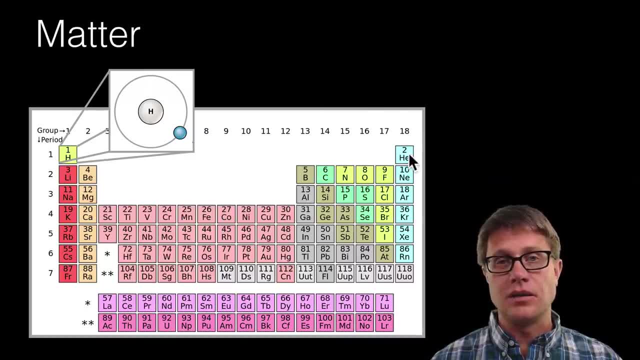 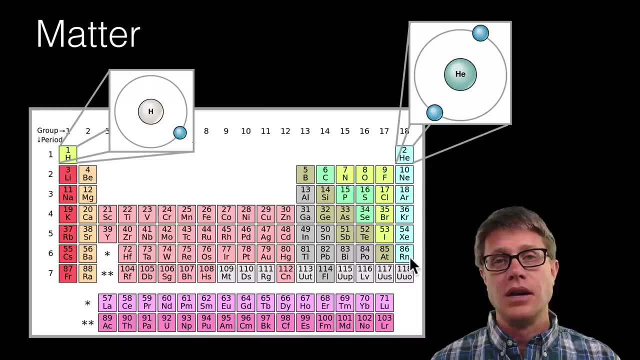 a single valence electron. If we were to go to helium, helium could have two electrons in this first shell And since it has two, it is incredibly stable. So is everything else right here. If we were to grab an important biological atom like carbon, it is going to. 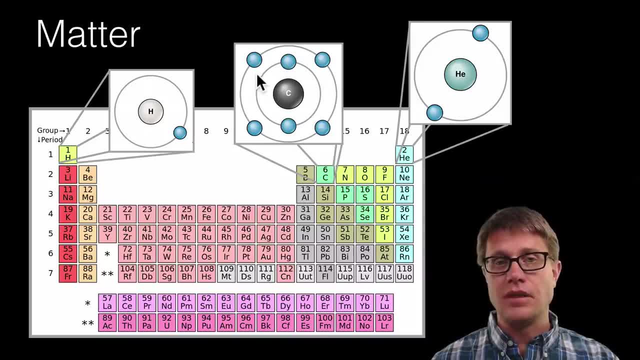 have four valence electrons, Two on the inside, four on the outside, So it is kind of the Lego block. We can build so many complex molecules off of that. And these are all through covalent bonds. And so if we look at methane, for example, methane is one carbon, four hydrogens We 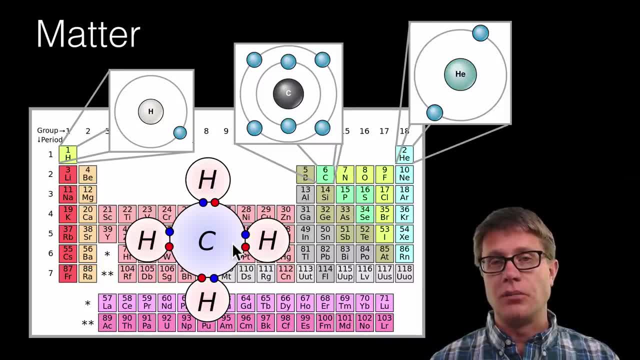 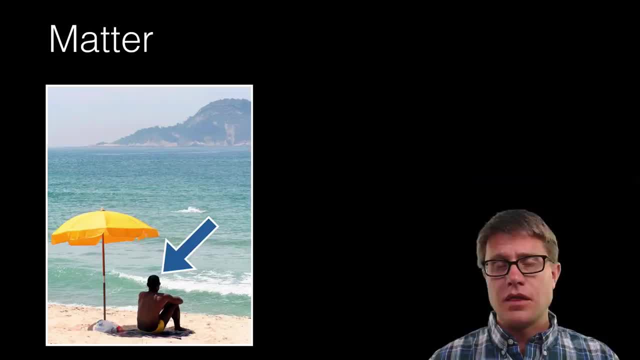 are sharing those electrons around the outside, So we have an incredibly stable molecule, And so the atoms we have on our planet are going to differ depending on where we are. So if we are looking at humans, think about this for a second. What are most of the atoms? 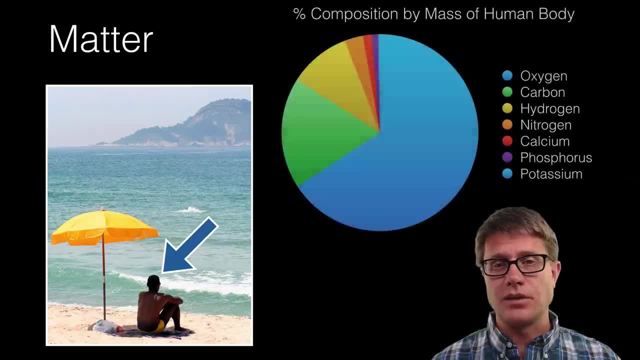 in a human going to be. Well, let's break it down by percent composition. We are mostly made of water, And so it is mostly going to be oxygen and hydrogen. We are built out of carbon, Hydrogen is made up of hydrogen and hydrogen is made up of hydrogen and hydrogen. 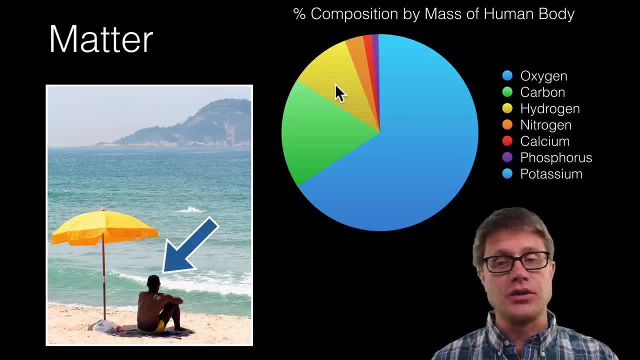 Hydrogen is so low because it has such a small mass. We are also going to have nitrogen, calcium, phosphorus, But in general we are going to be made by mass of oxygen. If we were to look at the water, so the sea water right here- what is most of that We could? 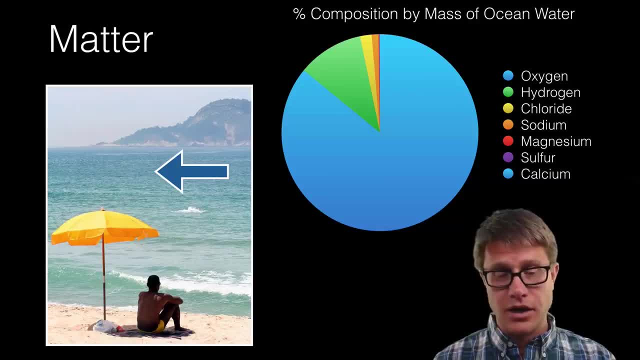 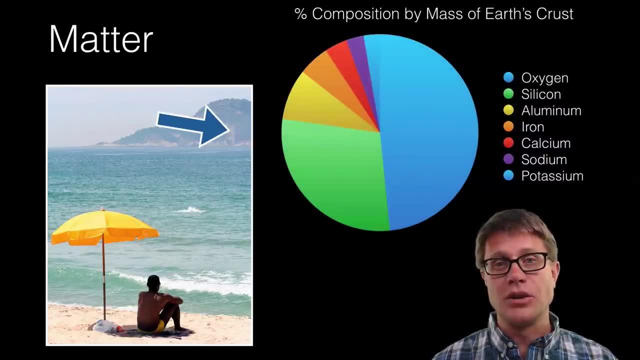 break it up this way, It is mostly going to be oxygen as well. It is mostly made of water. We are also going to have salts like sodium and chloride, But it is mostly made of oxygen and hydrogen. If we look at the rock, what is the rock? mostly made up of Oxygen. Now, 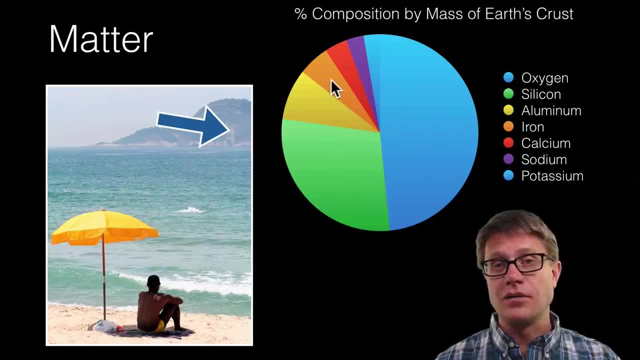 there is going to be silicon, We are going to have hydrogen, We are going to have oxygen, We are going to have aluminum and iron, But in general it is oxygen And if we look at the atmosphere, that is going to mostly be nitrogen, But we are also going to have a. 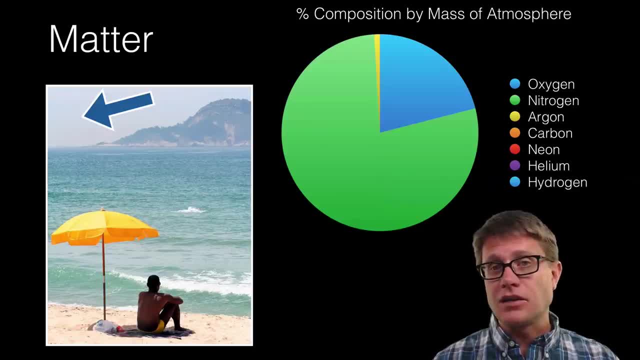 large amount of oxygen there as well, and other trace elements, And so the oxygen in the atmosphere can eventually become oxygen in the rock, It can be oxygen in the water, It can be oxygen in you. It has to be recycled because we are not creating new atoms on our planet Other. 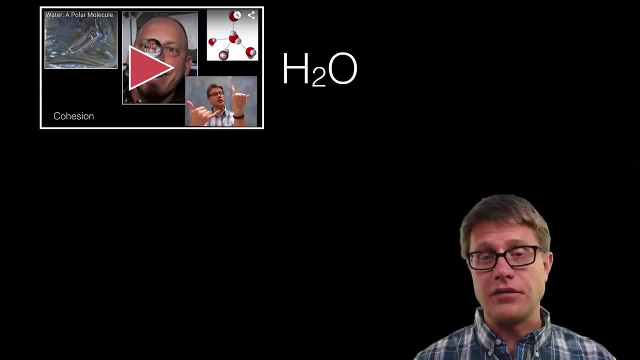 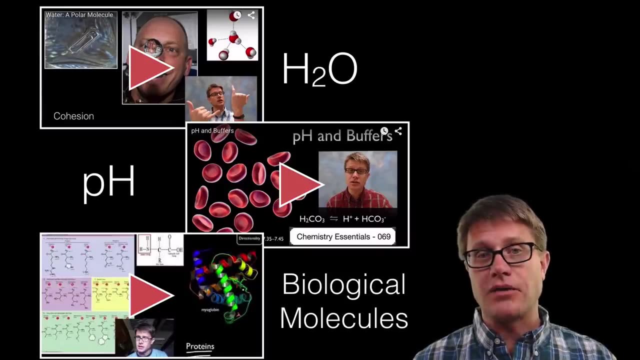 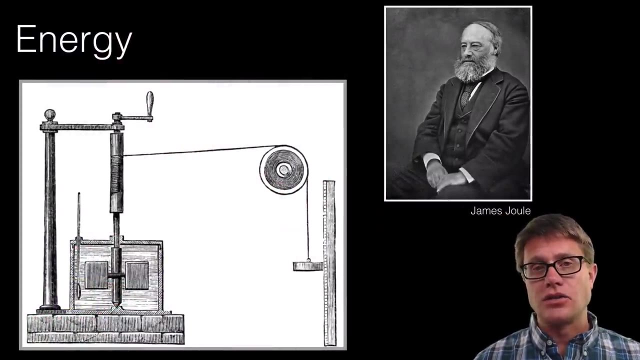 important parts of this course will be understanding how water is polar and that affects its behavior. OK, now we have h in such conditions as water, So we are able to understand what might actually happen with oxygen. Thank you, pr0. a joule. Now, when you talk about energy generally, you are going to hear things like watts, What? 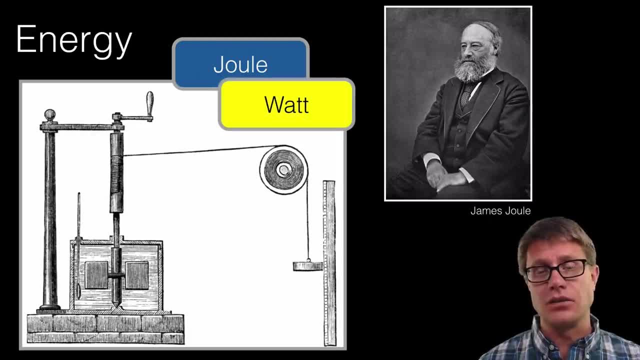 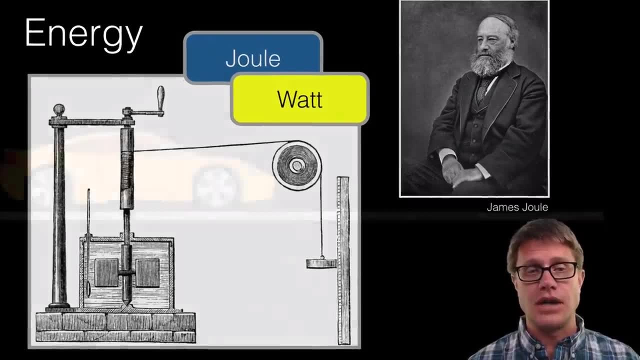 is a watt. A watt is going to be a joule per second, So it adds time. So if you are talking about kilowatts, we are measuring the amount of energy that is being used over a given period of time. Understanding the laws of thermodynamics is incredibly important, So 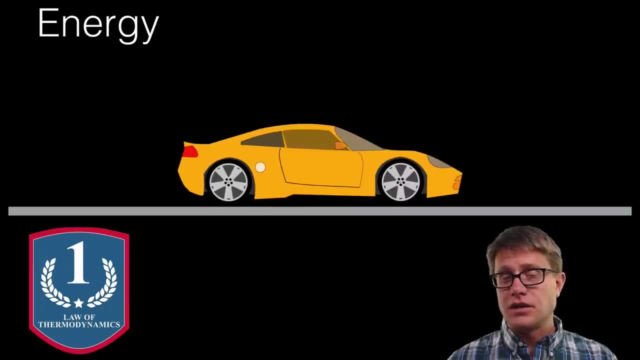 if a car moves from here to here, it is converting energy. We are not creating energy, We are converting it from one form to another. So where was the energy before it was in that motion of the car? It was in the gasoline Before then. it was in crude oil Before then. 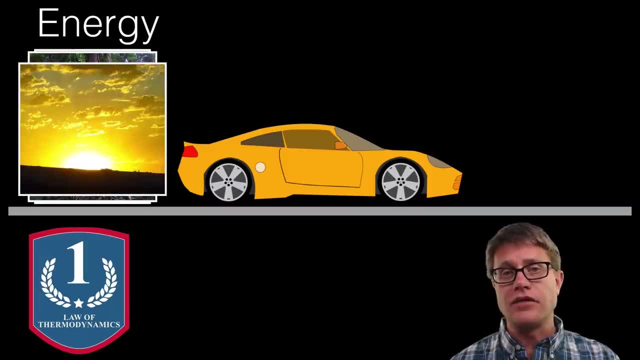 it was in an ancient rain forest. Before then it was given off by sunlight and used by that rain forest through photosynthesis. But we are not creating new energy. We cannot create or destroy energy. That is the first law of thermodynamics. The second law deals more. 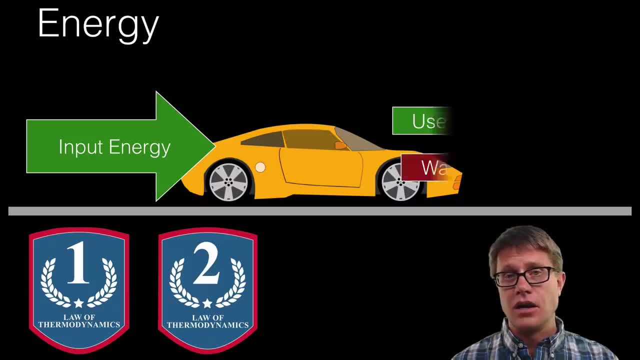 with systems. So we are going to have inputs into the system of the car And then we are going to have outputs And if we look at the amount of energy that goes into the car, we can think of that gasoline, the energy in the gasoline itself. we are using some of that energy for the kinetic 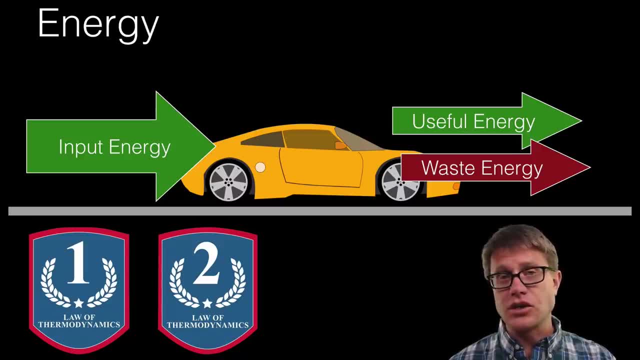 motion of the car. But we are also losing some of that energy in friction and heat and sound. And so what the second law of thermodynamics talks to is that at each interaction, at each point along that pathway, we are losing some of that useful energy. It is eventually becoming 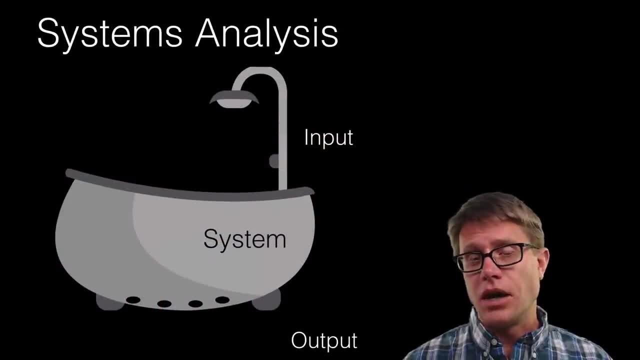 heat, which is non-usable on our planet. And so understanding this balance and understanding this system is the area of systems analysis, And this model works well. Think of it as a bathtub that has holes in it. You have got input and then you have got output. And if 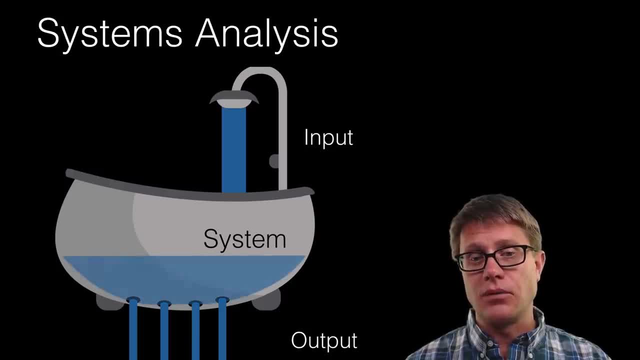 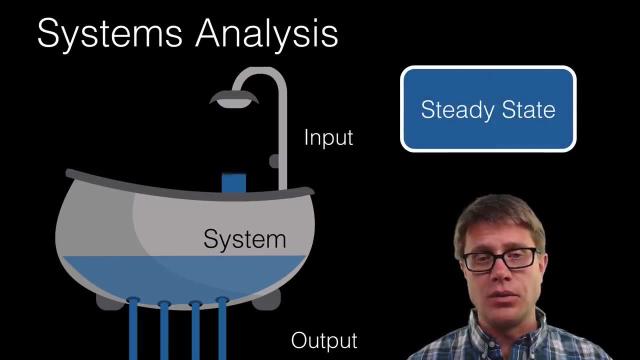 the amount of input matches the amount of output, then we are at what is called steady state. if we could see that. But what happens if we have an increase in inputs or an increase in outputs? What we can do is we can lose that steady state, And maintaining that is. 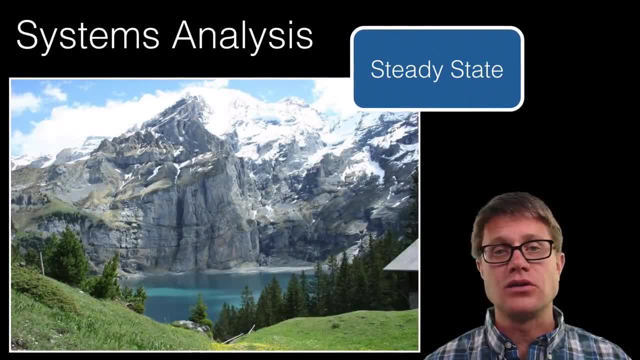 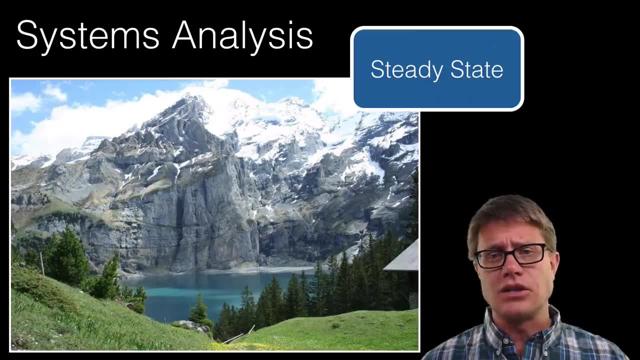 feedback loops. And so if we look at a real system on our planet- Swiss Lake- and we are going to find that the level of the lake is going to be steady state, And in nature, we find that almost all systems in nature are going to be steady state. So they are going. 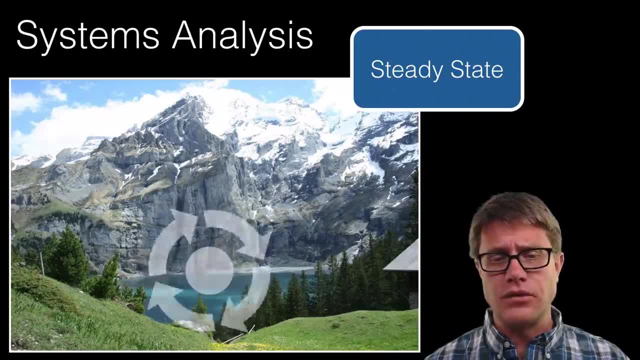 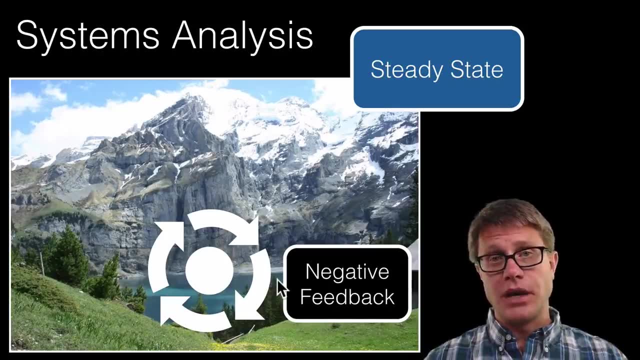 to stay at the same level. Well, how do they do that? They do that through feedback loops. And so, if you think about it, as we melt the snow, as we increase the amount of water in the lake, the level goes up. We might have more drainage, and that is going to keep the 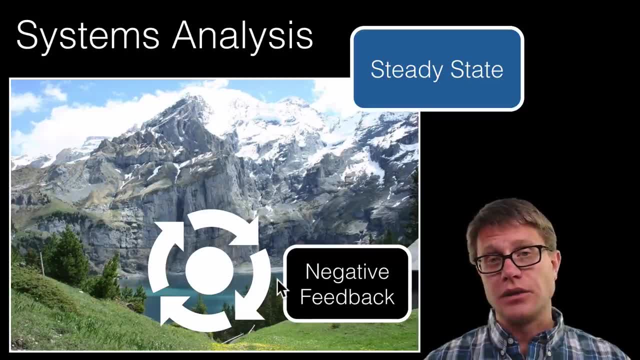 level the same. What else might happen? Since the lake is really large, we are going to have more evaporation off that surface area and the level of the lake is going to go down. Now we have a smaller surface area. there is less evaporation. now the level of the 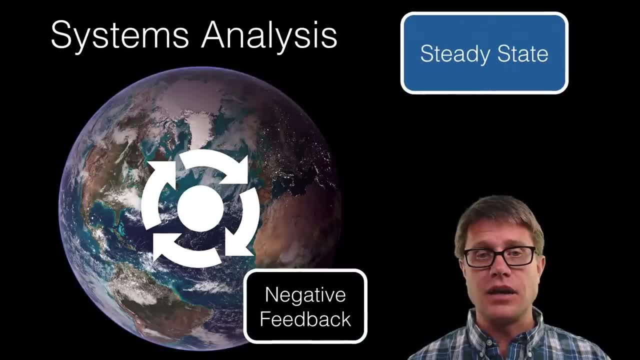 lake is going to go up, So that is a negative feedback loop. We could look at that at the level of the earth system as well. And so the earth is being heated, We are increasing greenhouse gases, We are increasing the temperature on our planet, And so there is a negative 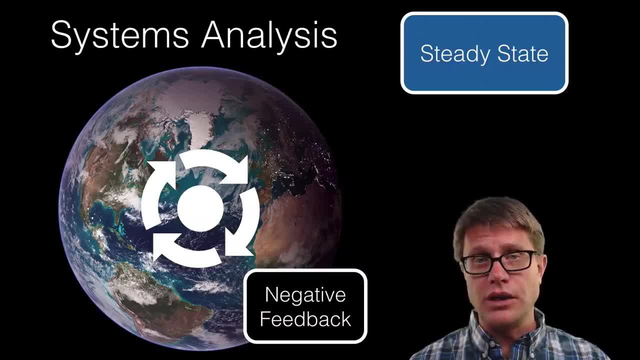 feedback loop that takes care of that. As we heat up the planet, there is more heat on the planet. What happens? We lose more of that heat to space, And so that is a negative feedback loop. The problem is that we also have positive feedback loops, So we have negative feedback. 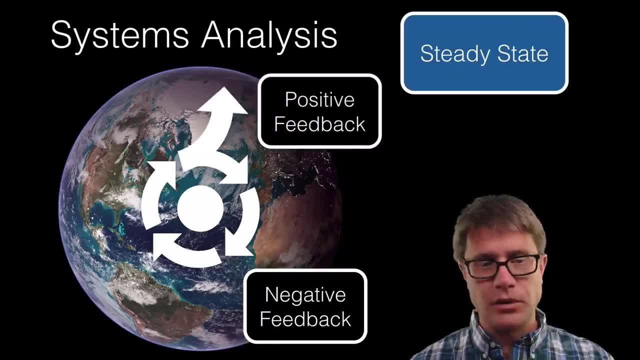 loops. We have negative feedback loops. We have positive feedback loops. We have negative feedback loops. We have positive feedback loops. We have positive feedback loops working on the planet right now. So an example: if we heat up the ocean, what happens? We are. 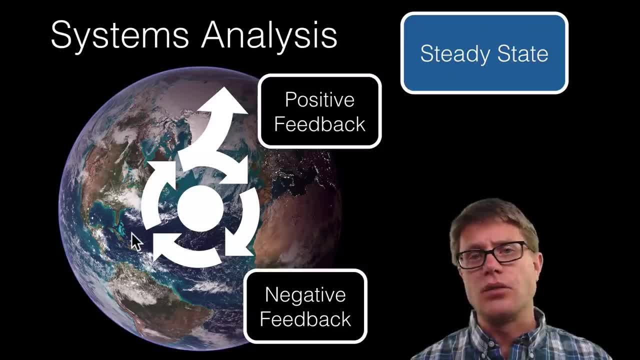 getting evaporation off the ocean. That creates water vapor, And water vapor is an incredible greenhouse gas. What does that do? It heats up the earth, which creates more evaporation of water and more global warming. Another example: we could look at this white area. 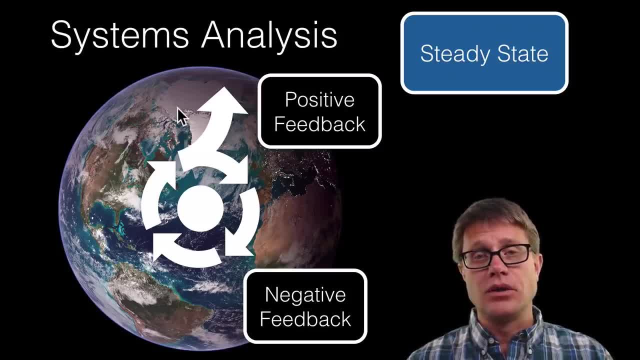 up here. So if we have a lot of ice that has a high albedo, It reflects a lot of the light back into space. What happens as we start to melt that ice? Then there is less albedo, We are absorbing more of that heat, And so we are. 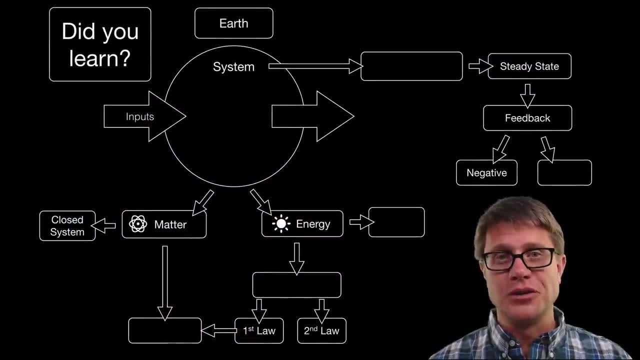 increasing the temperature. And so did you learn the following. I would pause the video right now and try to fill in the blanks, But I will show you what it all means, And so we can think of, remember the earth as a system. It has got inputs and outputs. We